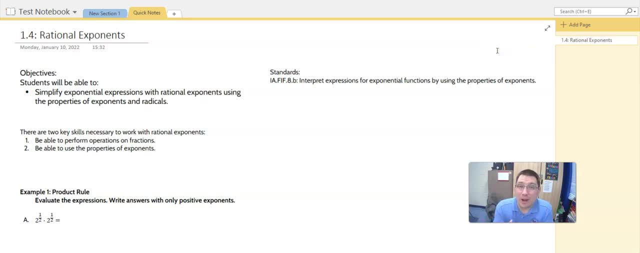 Hey there y'all. Today we're going to look at 1.4, on rational exponents. In this section, our objective is to be able to simplify exponential expressions with rational exponents using the properties of exponents and radicals. We're still under the same standard of being able to express exponential functions by using their properties of exponents. 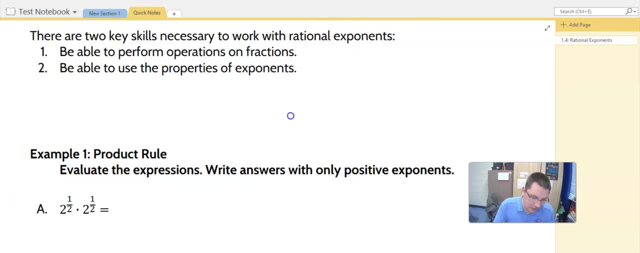 And so, first off, there's two key skills we need to talk about that are important to solving and working with rational exponents. The first is we need to be able to work with fractions. We need to be able to add fractions, subtract fractions and multiply fractions. 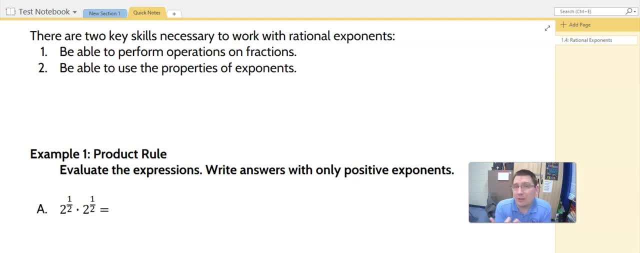 And we also need to be able to use the properties of exponents that we talked about in 1.3 and also the properties of radicals that we talked about in 1.1 and 1.2.. And so let's look at a few examples here of how we work with rational exponents. 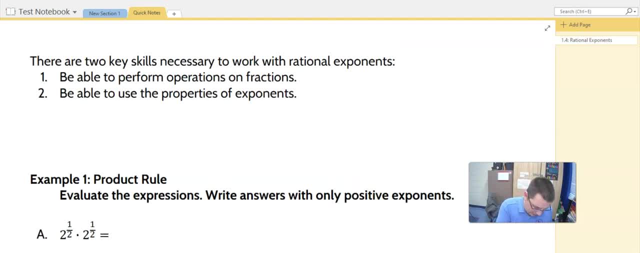 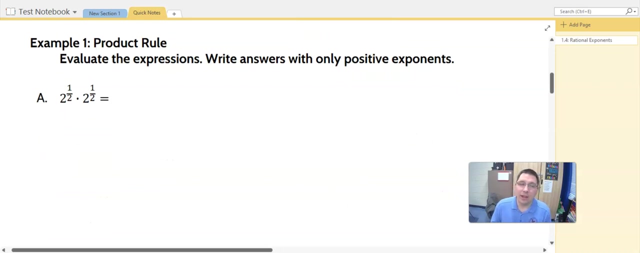 And that word rational. again, remember that word rational means that we are talking about fractional right Because, remember, the word ratio is a number that's written as a fraction right, And so fractional exponents. And so, looking at example 1a, we want to be able to evaluate these expressions and write them with only positive exponents. 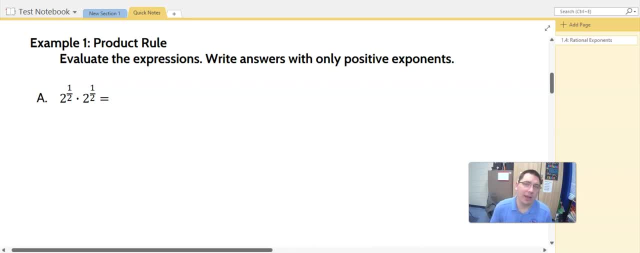 And so we have 2 to the 1 half times 2 to the 1 half, And so, remember, that's our product rule, and so the base will stay the same at 2.. And our powers are going to add: So 1 half plus 1 half is 2 halves or 1 whole. 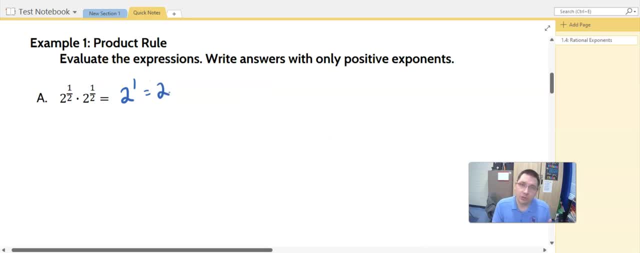 And so we get 2 to the 1st or just 2.. And we can do that with any power right. We can do it with 1 half plus 3 halves, We can get 4 over 2 and reduce it down to 2. And so we can do it with any fractions. 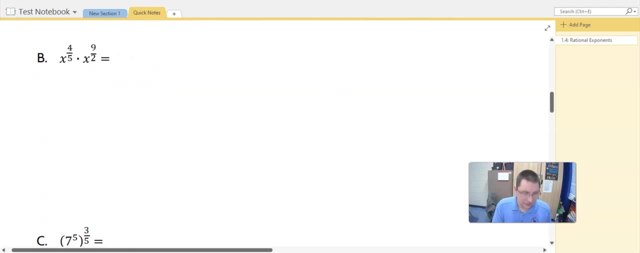 As we look at example b, we've got x to the 4 fifths times x to the 9 halves. Now these two fractions aren't going to add. Adding them together is easy, And so we might want to come out to the side here and do 4 fifths plus 9 halves. 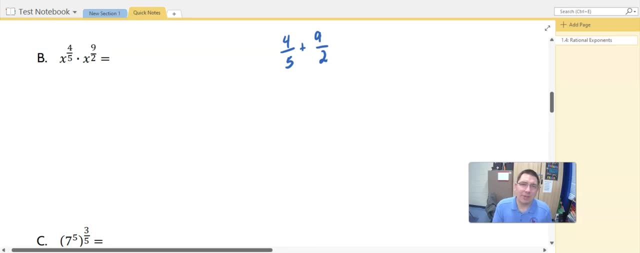 And remember, to add fractions, we need to have a common denominator. And so you know, your middle school teachers might have taught you a couple different methods, but remember the key to adding fractions is to have a common denominator. And so what would that common denominator be for 5 and 2?? 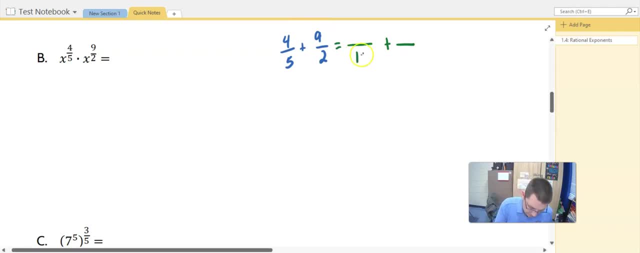 Well, if we multiply 5 times 2,, we get 10.. And so multiplying the denominators will always give us a common denominator, but it won't always be the least common denominator. Remember, the least common denominator would be the first number that both numbers could multiply to. 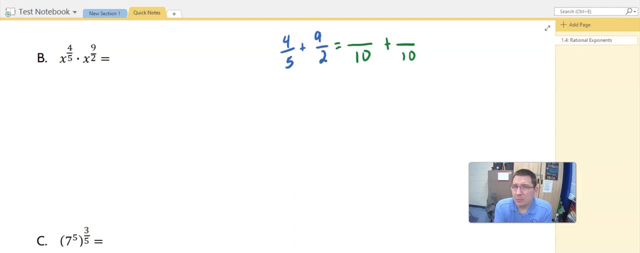 And so for 5 and 2, that is 10.. But what if we had 6 and 4?? Well, 6 times 4 is 24, so we could use that as our denominator, But we could also reduce that down. 6 and 4 also multiply to 12.. 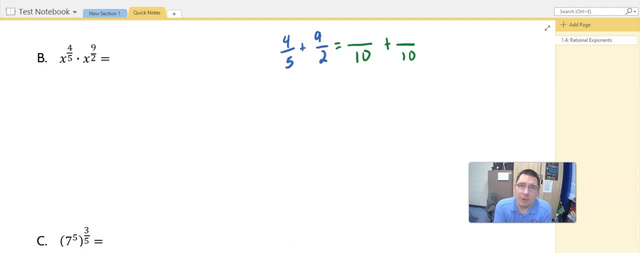 And so that would be the least common denominator. So that would be the least common denominator of those two numbers. Alright, so coming back to this, 4 fifths plus 9 halves. Well, remember that when we multiply this 5 to get 10, we multiplied it by 2.. 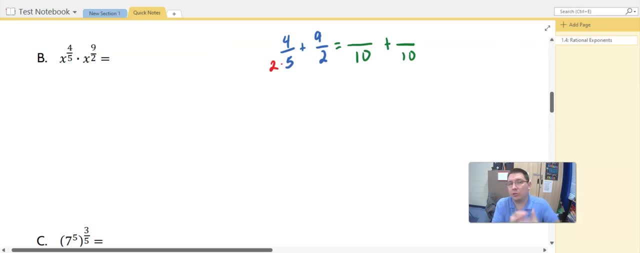 But whatever we do to the denominator of a fraction, we also have to do to the numerator, And so the 4 is going to get multiplied by 2 and give us 8.. And then we look at the second fraction: 9 halves. Well, we multiply the 2 by 5 to get us 10.. 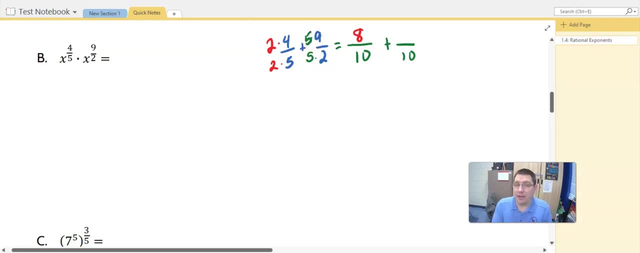 So we're going to multiply the 9 by 5 to give us 45. And then we're able to add those two fractions together. And remember to add fractions. we're going to add the numerators and keep our common denominator. 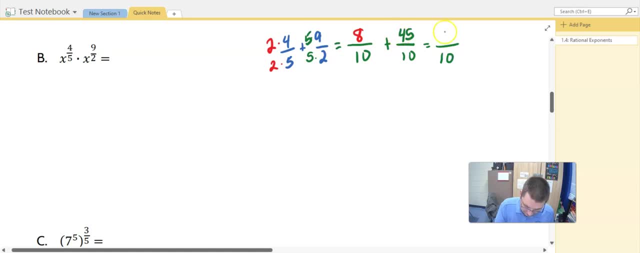 So our denominator is 10.. 8 plus 45 is 53. And so this is going to be x, because we keep our base with this property. So we're going to multiply the 2 to the 53 over 10 power. 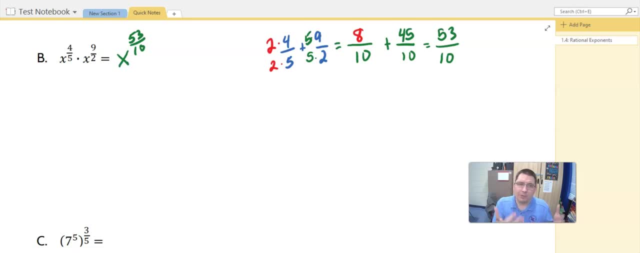 Now again, that seems like a crazy power, But the property is what it is right. We're going to add these fractions and get our new rational exponent. Let's look at example C. We have 7 to the 5th to the 3 fifths power. 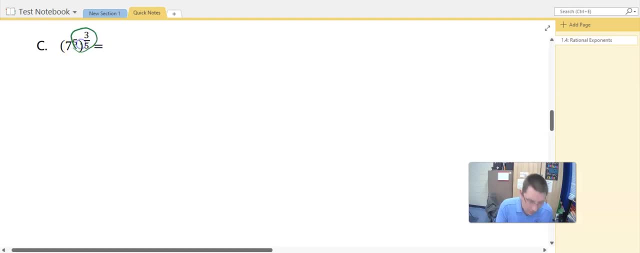 And so, since we are power to power, remember we're going to multiply those two powers. So I want to come off to the side and do it as scratch work. So 5 times 3 fifths. Well, remember to multiply fractions. we multiply straight across. 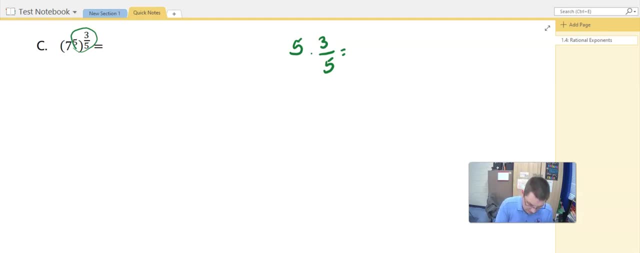 Numerators to numerators, denominator to denominator, And so we can put this 5 over 1.. So we're going to get 5 times 3, 15.. 1 times 5, 5.. And so 15 over 5 reduces to what? 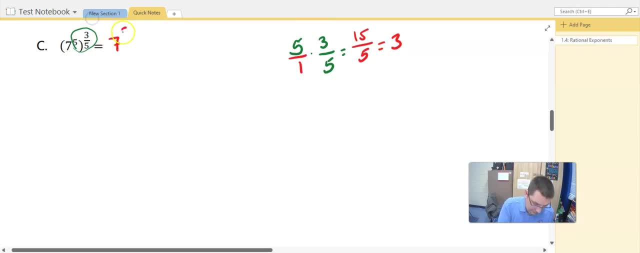 3. And so this is going to give us 7 to the 3rd power, And again, for what we're working on here, we can leave it 7 to the 3rd. If we actually need the value, we can rewrite it. 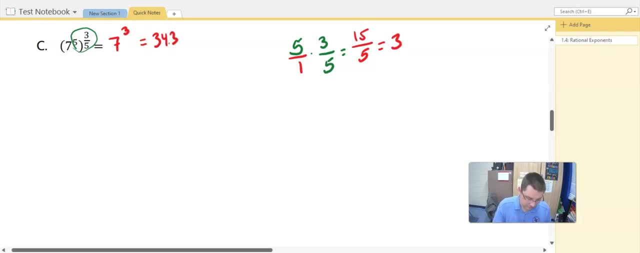 And 7 to the 3rd is 343.. Let's look at example 2, where we're talking about converting from rational exponents to radicals, And so remember this goes back to section 1, relating rational exponents to radicals. 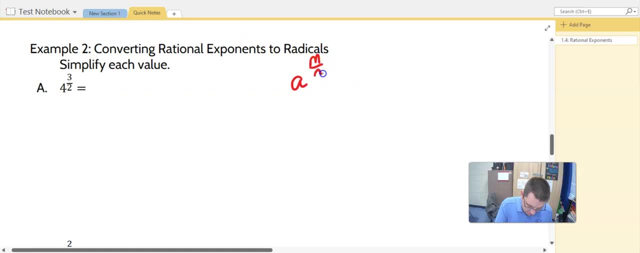 And so if I have a to the m over n power, we can convert that to a radical. The a will be our radicand the part inside the radical, And then our index is the denominator of that exponent. And so, again, the denominator is the index. 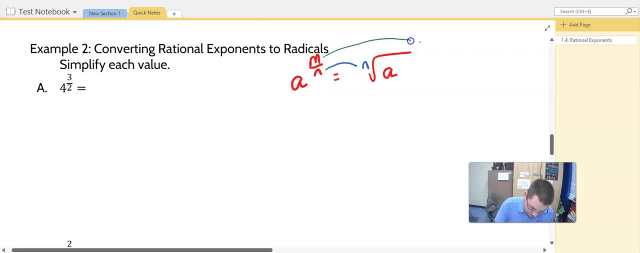 And the numerator, the m, in this case, will be the power outside, And we'll put that around in parentheses Now you might also see it written: with the power inside, So the nth root of a. With the power inside, So the nth root of a, to the m. 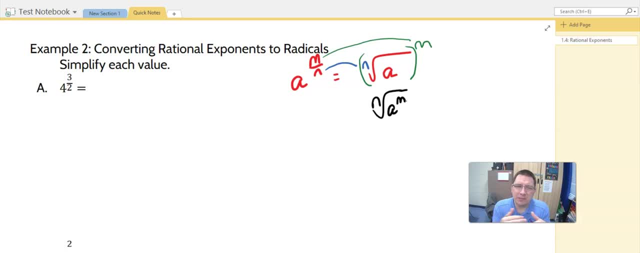 That is another way to write it, But for what we're going to be doing with these type problems, we're going to want to have that power on the outside, Because we're going to want to simplify the radical part first, which will give us a smaller number, typically. 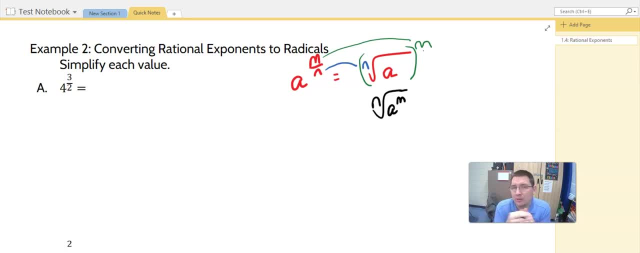 and then raise it to the power that is requested. And so let's look at example a: 4 to the 3 halves power. Well, we're going to rewrite this as a radical, And so put your radical And the 4 will go inside. 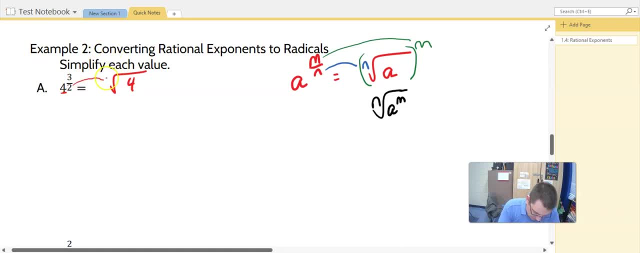 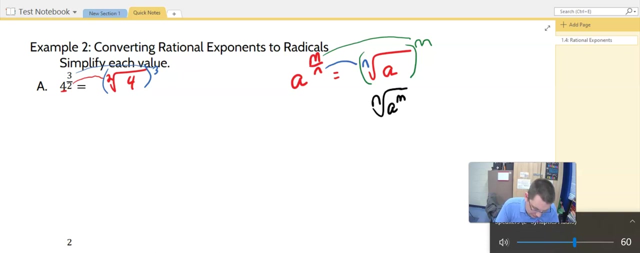 The denominator of this power will be the index. So we're doing the square root, And then the numerator of this power will be the power, And so we're going to reduce this part inside. first, What is the square root of 4?? 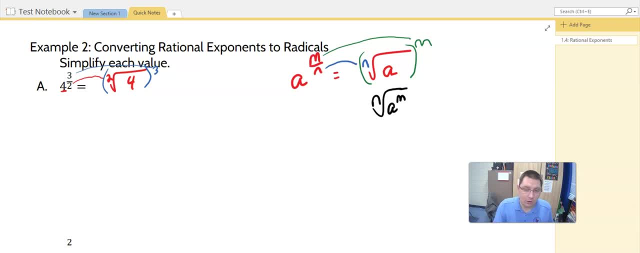 Well, what times? itself gives you 4, right. So the square root of 4 is 2.. And so 2 cubed. well, 2 times 2 is 4, times another 2 is 8.. And so the final answer here is just 8.. 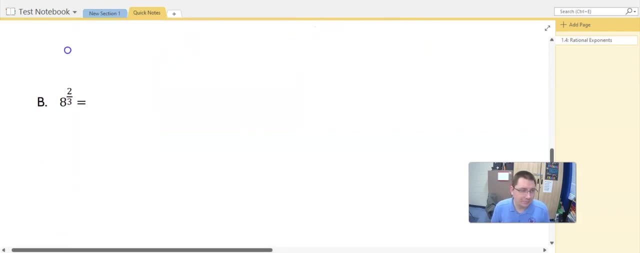 Let's look at example b: 8 to the 2 thirds power. So again, we're going to convert this over to a radical so we can simplify it by piece. And so we're going to write our radical. The 8 will be the number inside the radical. 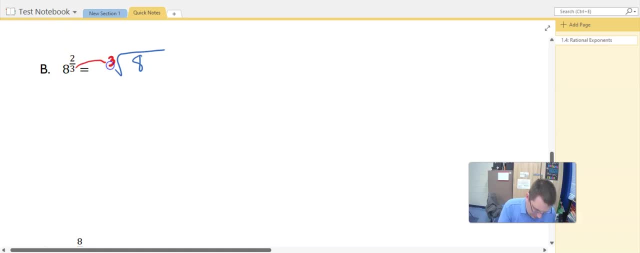 The 3 in this case is the index And the 2 is our power out back. And so we're going to ask ourselves: what is the cube root of 8?? Well, what times itself, times itself, will give us 8?. 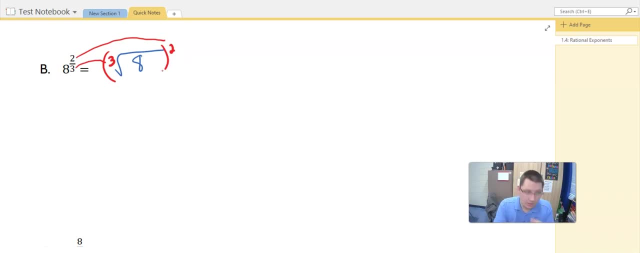 2 times 2 times 2 is 8.. And so we're going to get 2 squared, And 2 squared is what? 4.. And so we see that there, And so, again, we want to take these three pieces. 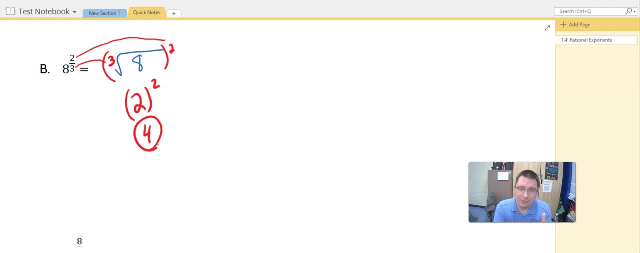 the three components of this rational exponent- the base, the numerator and denominator of the power- and put them each in their own place as a radical and be able to simplify it. Let's look at example c. We have 32 to the 8 fifths power. 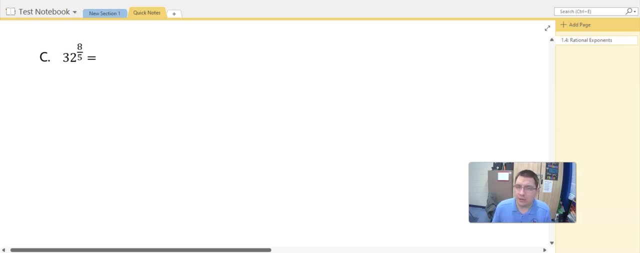 So a little bit larger number here and larger power and denominator, And so again we'll put our radical: The 32 will go inside, The 5 is the index And the 8 is our power. And so we have to ask ourselves: 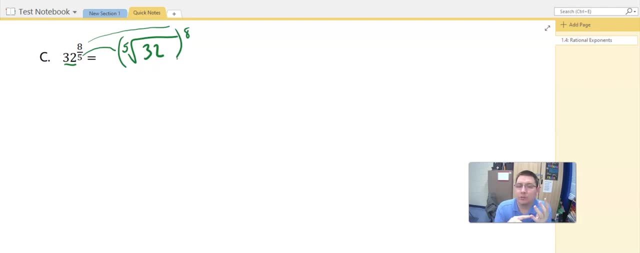 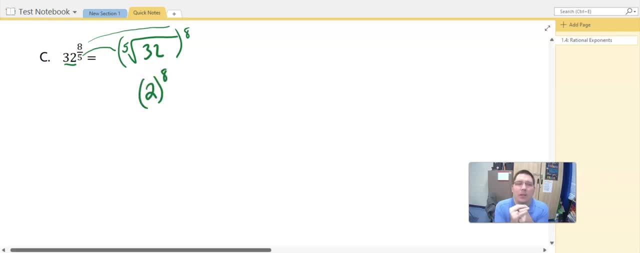 So this is going to be 2 to the 8th, And so now I got to do all those 2s multiplied together. Well, we just talked about 5 of those together was 32.. So we just keep going. 6 is going to be 64.. 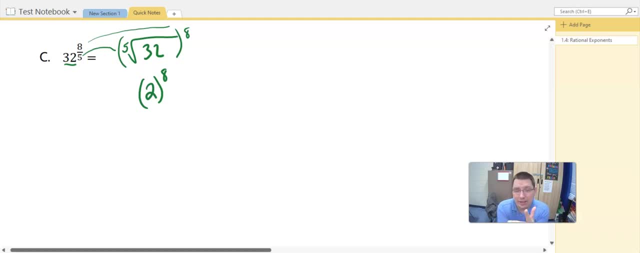 7 is 128. And 8 is 256.. So 2 to the 8th is 256. So we can get that value there. So again, we're going to use those powers to simplify this to its own value. 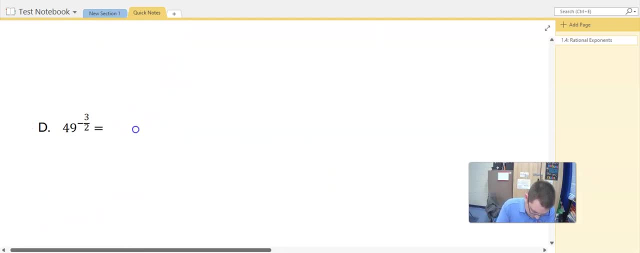 And let's look at d. We've got one more example here And we'll erase that part. 49 to the negative 3 halves power, So 49 to the negative 3 halves. Well, in this case we've got to deal with that negative exponent first. 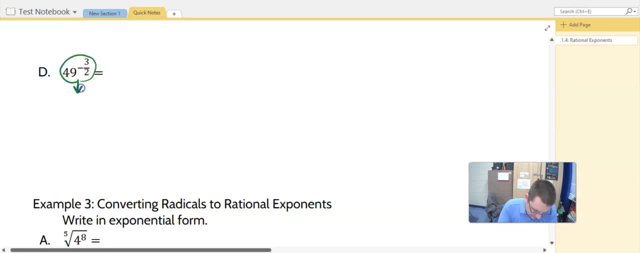 And so dealing with the negative exponent, all of this is going to go to the denominator and change that power from negative to positive, And so we're going to get 1 over 49 to the 3 halves power. And so now we'll deal with that rational exponent. 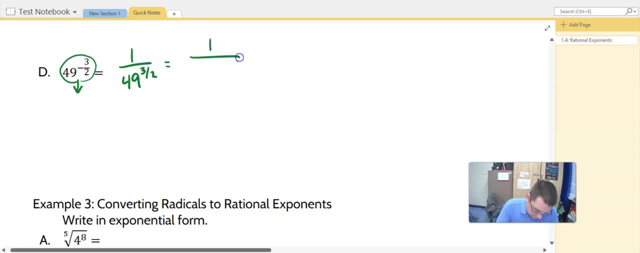 and make it a radical, And so we'll rewrite it. 1 over the square root, because that's our index of 49 to the third power. And so, again, we'll break this down piece by piece: The square root of 49.. 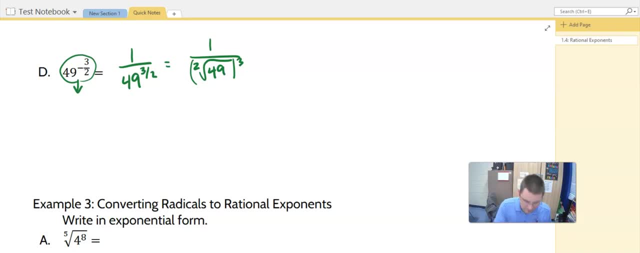 What times itself gives 49?? Well, that's 7.. And so we're going to get 1 over 7 cubed, And 7 cubed is 343.. So the final answer here is 1 over 343.. So we see how, with that negative exponent, 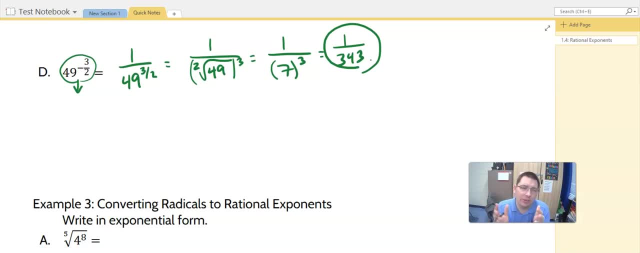 we still have to deal with it before we can change it from that rational exponent into the radical. Now, the big key here with all these problems is: I want you to be able to convert it from rational to radical Because, yeah, you could do this on your calculator, right? 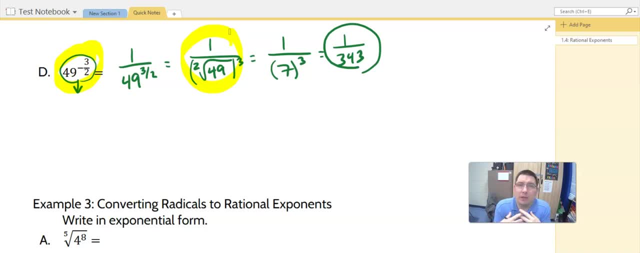 We could type in 49 to the negative 3 halves and it would give us the decimal of what 1 over 343 would be. But being able to convert from 1 to 3 to the other is important for solving equations And that's what we're getting to. 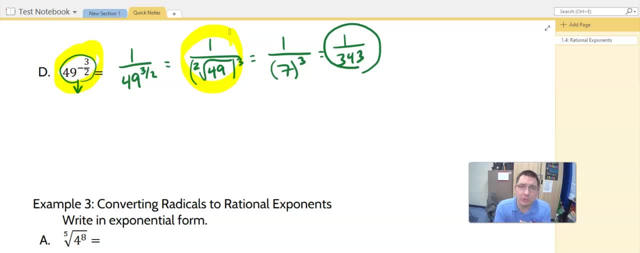 as we get further through this unit and into other units, We need to be able to use these power rules to simplify equations, And so that's where this skill is important. Let's go ahead and look at example 3.. And we've got a couple examples here. 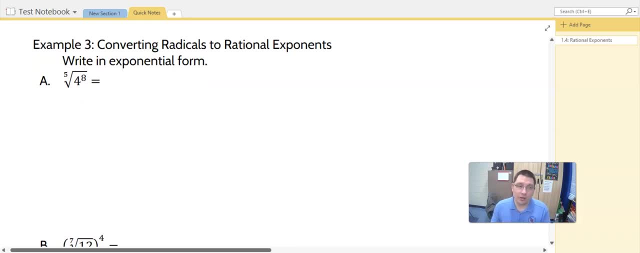 of converting the other direction. We're going to convert from radicals to rational exponents, And so these. we're not going to want the decimal right Because, like the fifth root of 4 to the eighth, it's going to be an ugly decimal. 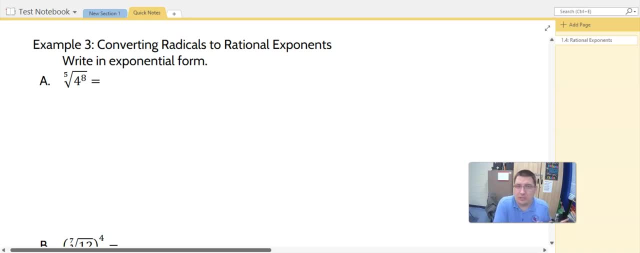 because the fifth root of 4 is one point, something really small, right? Because if I'm taking the fifth root, the fifth root of 32 is 2, so we're something like 1.1.. So we're just converting these. 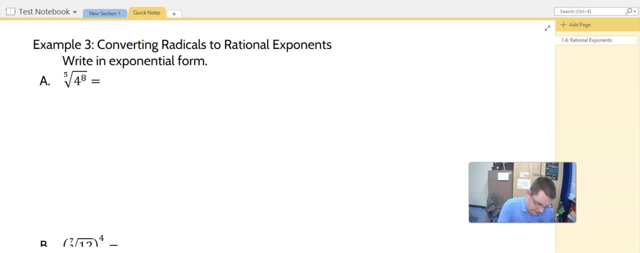 to be able to convert from one to the other. Again, it's just practicing that skill, And so we want to convert this over. So remember what goes where. Well, the 4 becomes the base of the exponent, And then we're going to have our power. 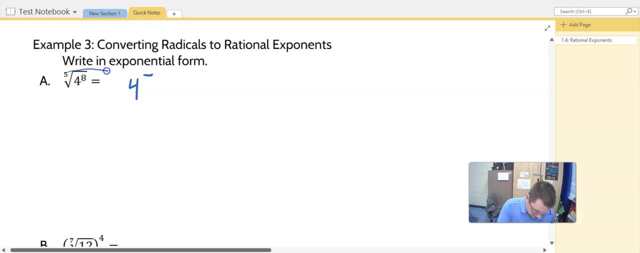 which is a fraction, And remember that the index is our denominator and the power is our numerator. And so we end up with 4 to the eight-fifths power. And again, we're not looking for the decimal here, We're not looking to simplify this. 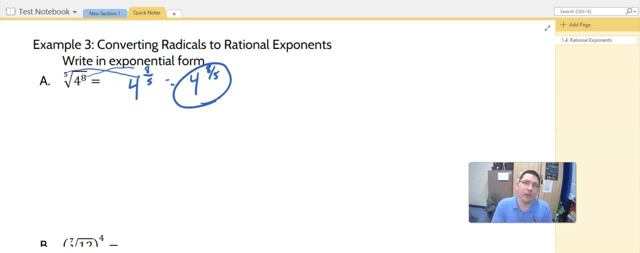 We just want to convert it from the radical form into the rational exponent form. And so there's one more example we're going to look at real quick: The seventh root of 12 to the fourth power, And so, again, we're converting this over. 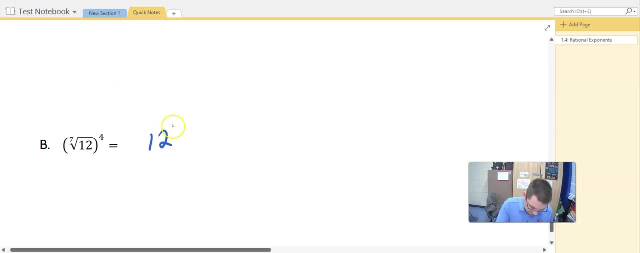 So 12 is our base. Think about what goes where for our fractional exponent. The 7 is our index, so that'll be our denominator. The 4 is our power, and so that would be our numerator of the final power. And so this is 12 to the four-seventh power.